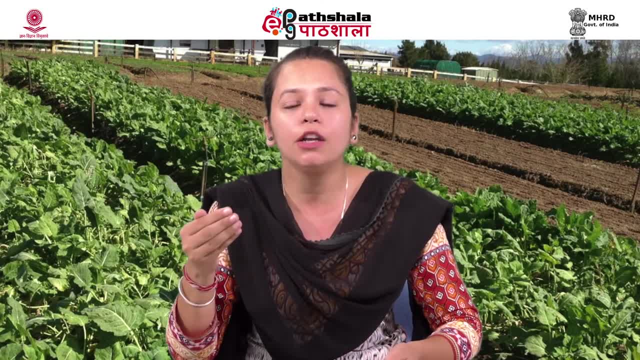 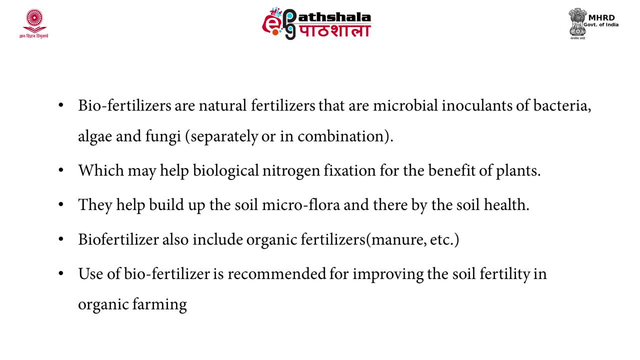 for the proper plant growth or you can say for increasing the yield of product. Biofertilizers are economic and eco-friendly. That's why most of the people they are moving further. they need biofertilizer to use for the enhancement of plant growth. The biofertilizers were initially 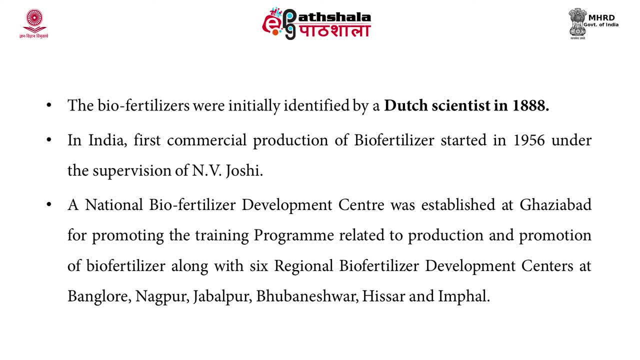 identified by a Dutch scientist in 1988.. In India it was first commercially. its production started in 1956 under the supervision of NV Joshi. A National Biofertilizer Development Center was established in by Indian government at the Ghaziabad for promoting the training. 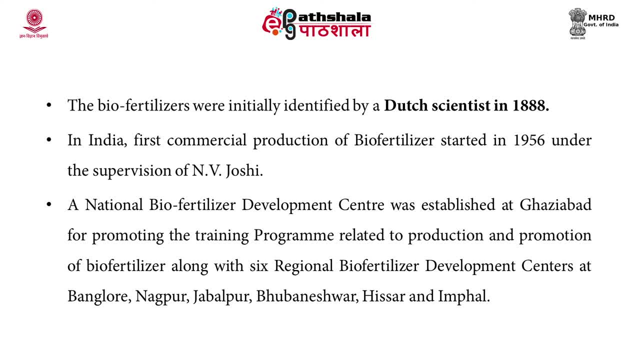 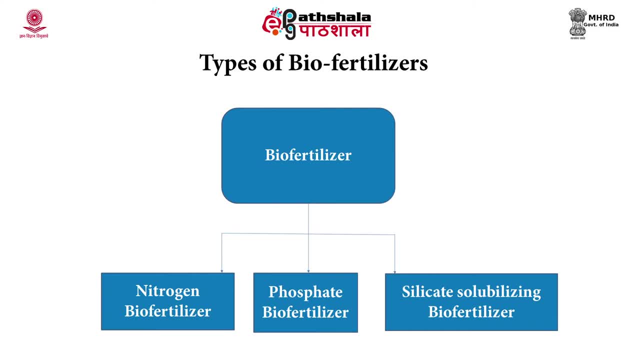 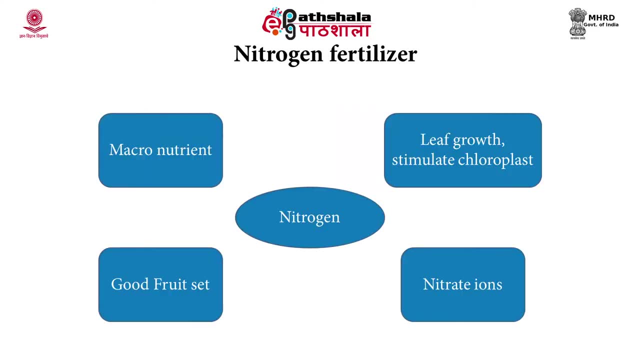 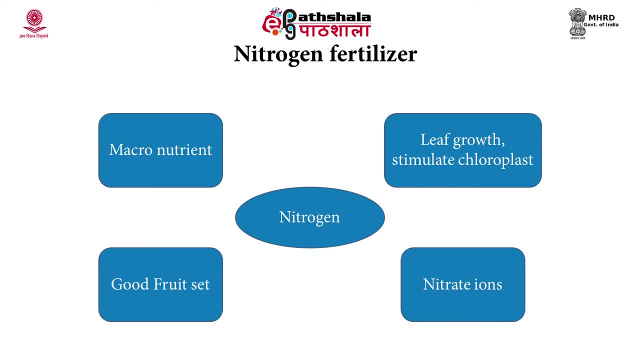 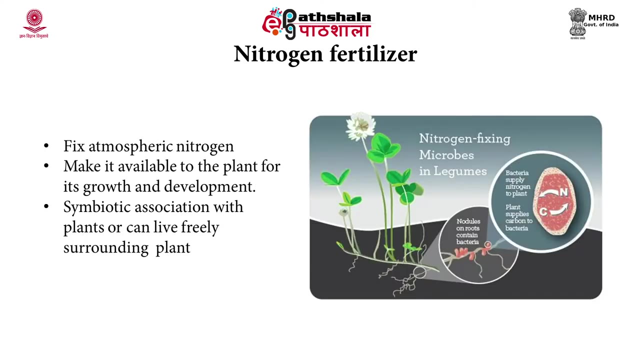 that is required by the plant for its leaf growth. it helps in stimulation of chloroplast chloroplast production. it enhances the fruit set. nitrogen is used by the plant in the in the form of nitrate ions. what these nitrogen fertilizers do? they help in fixing the atmospheric nitrogen. 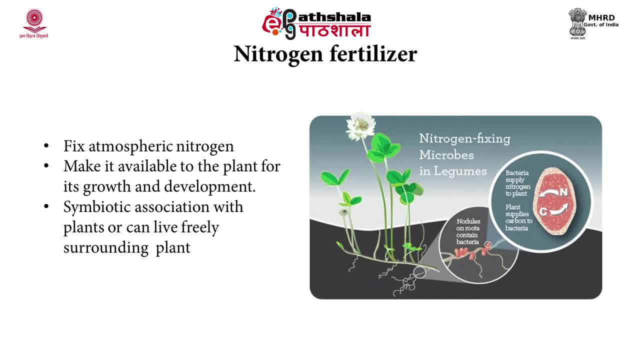 and making it available to the plant for its better growth and development. nitrogen fertilizers: it means the microorganism that are used as a nitrogen fertilizers. they are symbiotic, ly associated with the plants. what does? what is the meaning of symbiotic association? that means both. 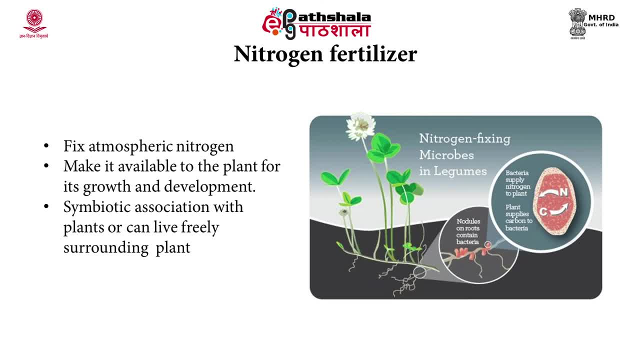 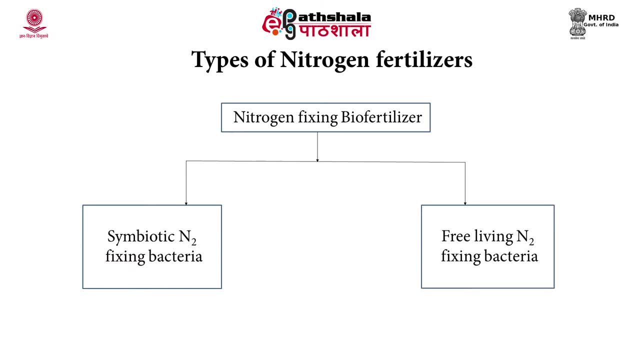 the partners are equally benefited. they they form a symbiotic association with the plant and can live freely around the plant. further, the types of nitrogen biofertilizer: nitrogen fixing biofertilizers are of two types. one is the symbiotic nitrogen fixing by bacteria and the other one is free-living nitrogen fixing bacteria. let's discuss about the symbiotic nitrogen. 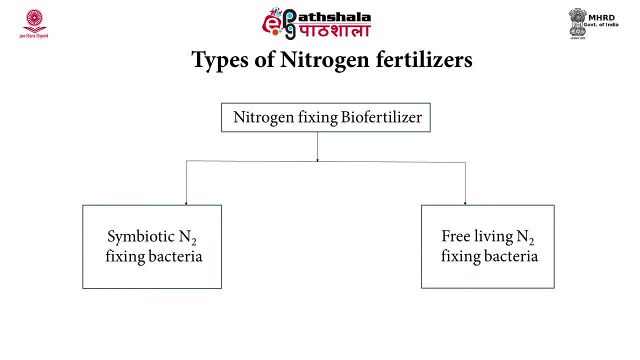 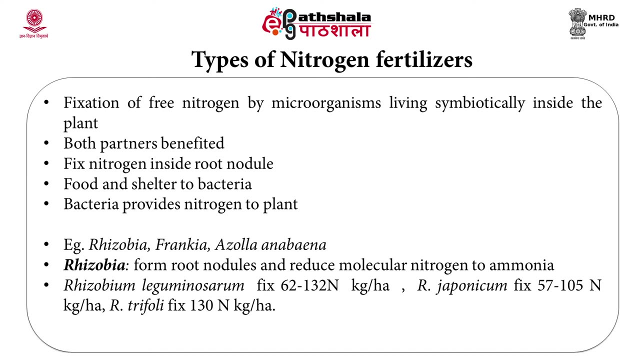 fixing bacteria. as I told earlier that what is symbiosis, it means the mutual benefit of both the partners. they help in fixing the free nitrogen by symbiotic ly living inside the plant. in this process both the partners are benefited. the whole process that the fixing of nitrogen by from the atmospheric nitrogen it undergoes inside the root nodules. 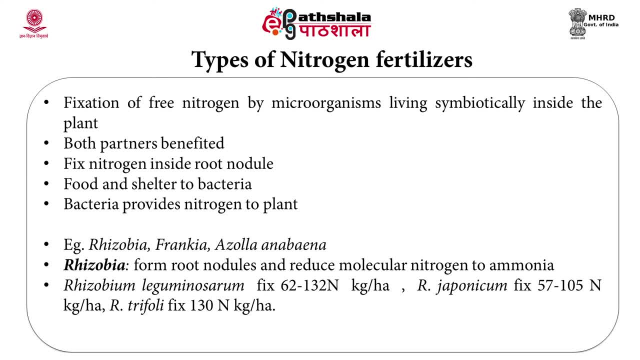 what the bacteria? bacteria they are getting food and shelter by living inside the root nodules and which in turn converts the atmospheric nitrogen into into the available form to the plant. examples of symbiotic ly fixing nitrogen bacteria are rhizobia francia, phytophthora and phytophthora. 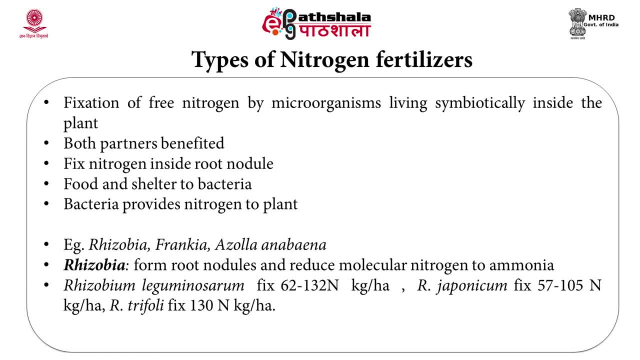 azolla anabina. we'll discuss these examples one by one. what is rhizobia? it is root nodules forming bacteria and it reduces the molecular nitrogen to ammonia. it converts the atmospheric nitrogen to ammonia and then that microorganism further make it available for the plant growth rhizobia. 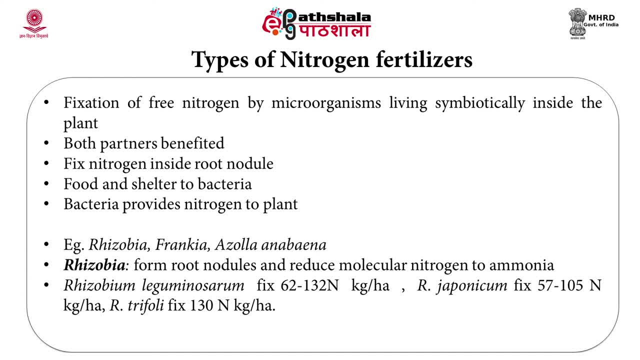 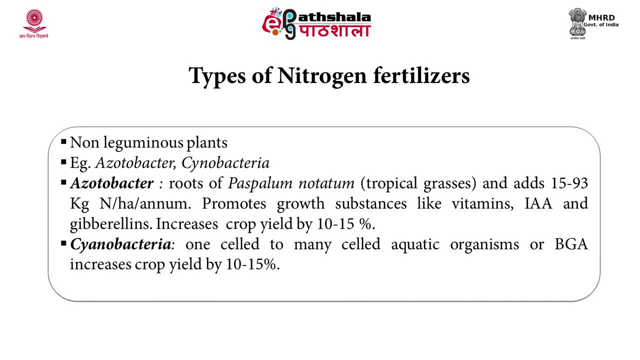 leguminosum fix 60 to 132 nitrogen kg per hectare. then azolla anabina, the type of symbiotic ly fixing bacteria. it fix the nitrogen in association with blue green alga. it helps in azolla, as we know that azolla is a free floating water fern. it fix the atmospheric nitrogen in paddy fields and also used. 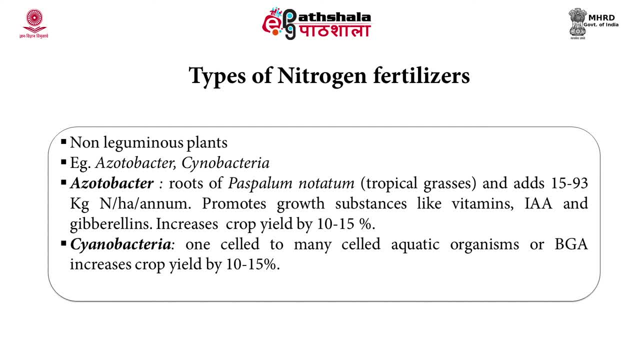 as a feed substitute for livestock azolla. biofertilizer, azolla anabina. the living formulation of azolla anabina as a biofertilizer: it increases the yield up to 10 to 20 percent in the paddy crop. also act as a biocontrol agent as it's a 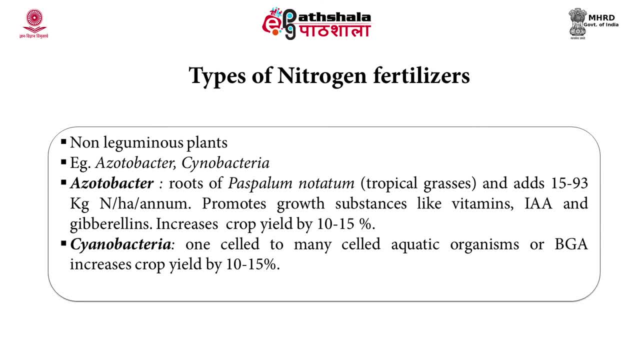 biocontrol agent. it increases the weed growth. the next is francia. francia is the genus of nitrogen fixing mycelial bacterium that is actinomycetes. it's symbiotic ly associated with the non leguminous plants we discussed earlier about the rhizobia. that rhizobia work in association with the root. 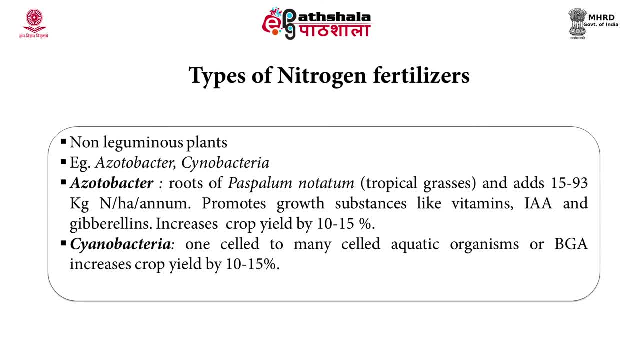 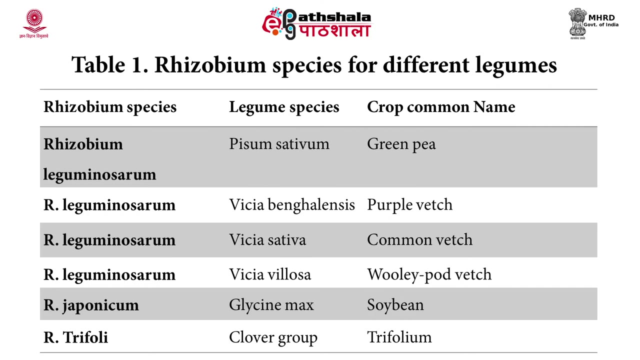 nodule plants, that is, leguminous plants, and francia. it is used it. it it goes under association with non leguminous plants. this francia is capable of infecting and non nodulating group of eight families, mainly woody plants, called as actinorhizol plants. table 1 describes the rhizobium species for different legumes, the- we can say the. 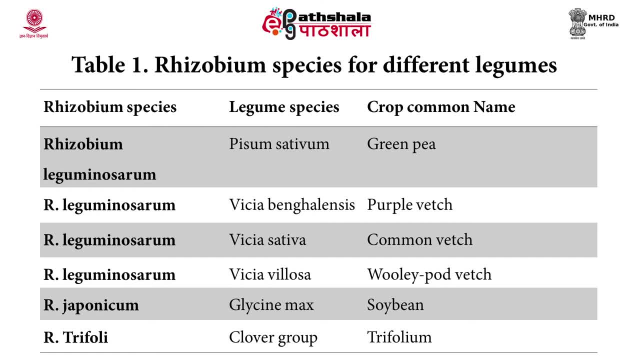 speciality or this the rhizobium species. they are particularly crop specific. for example, the rhizobium leguminous serum is used against only the woolly pod batch plant. rhizobium japonicum is used for the species named glycemic max. its common name is soya bean. 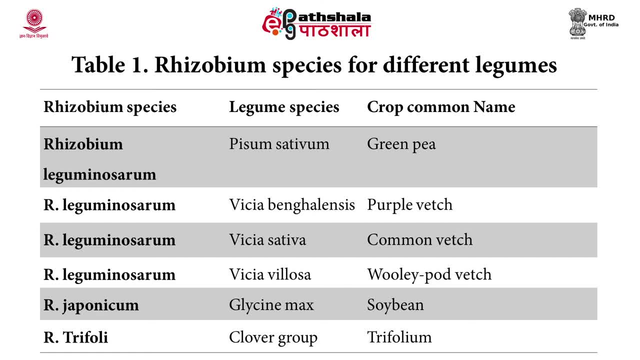 In that way, there are nine species that we have discussed in that we have mentioned in this table against rhizobium species and their target crop plant. We discussed about the symbiotic nitrogen fixing bacteria. now we will discuss about free living nitrogen fixing bacteria. 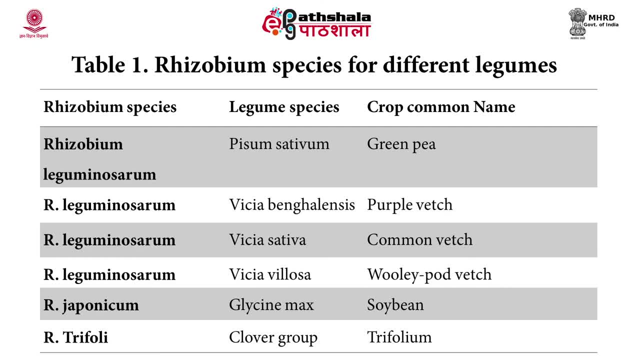 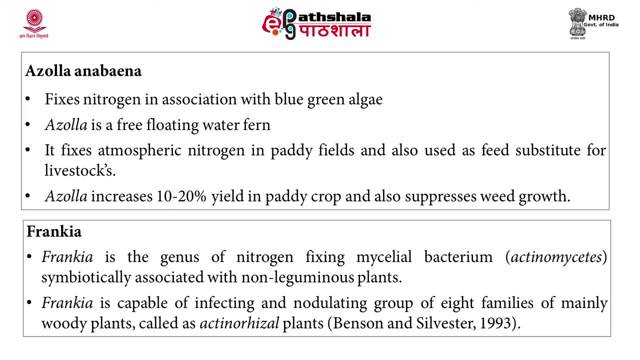 Rhizotobacter. it was found that it is found in the roots of Phosphonium notatum, tropical grasses, and adds 15 to 93 kg per hectare per annum of nitrogen to the plant and it helps in and promotes the growth of substances like vitamins, Indole acetic acid, which is an auxin. 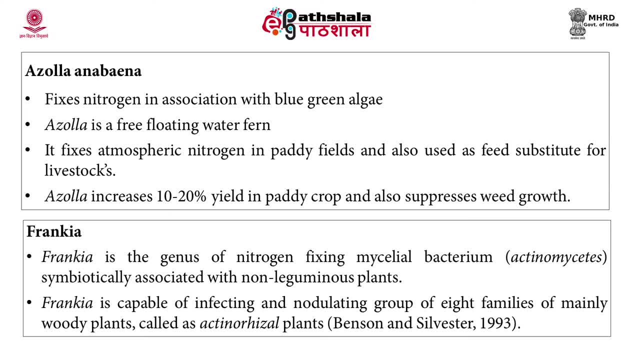 which further helps in enhancement of plant growth, And gibralin, Which increases the crop yields by 10 to 15 percent. Next is cyanobacteria. it. cyanobacteria is, or BGA, that is, blue green algae. it increases the crop yield by 10 to 15 percent. 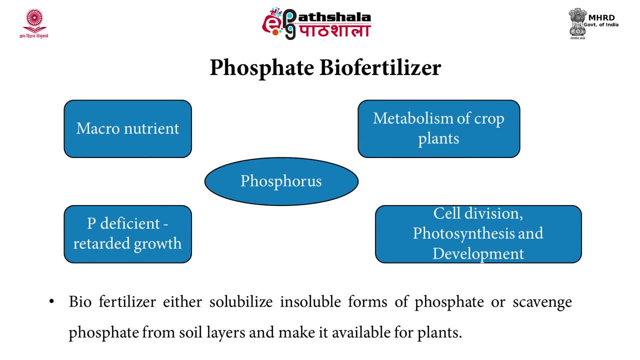 We discussed about the nitrogen fixing nitrogen bio fertilizers. now we will discuss about the phosphate bio fertilizers Similarly. first the why phosphorus is necessary. what role phosphorus play in the plant growth. Phosphorus is a macronutrient. it helps in metabolism of crop plants. its major role. 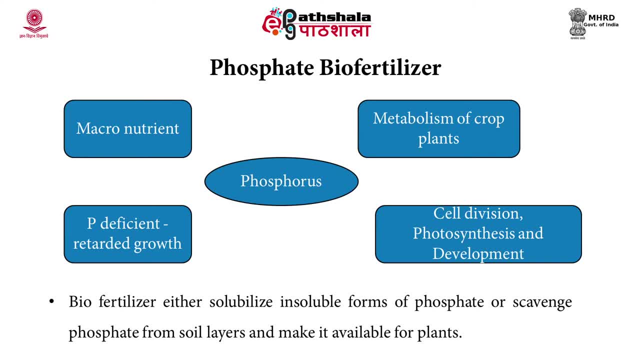 is in the cell division and photosynthesis part of the plant. If a plant is a phosphorus deficient, that is, P deficient, then it shows retarded growth. As I told you that it helps in cell division. if there is no cell division, there will be. 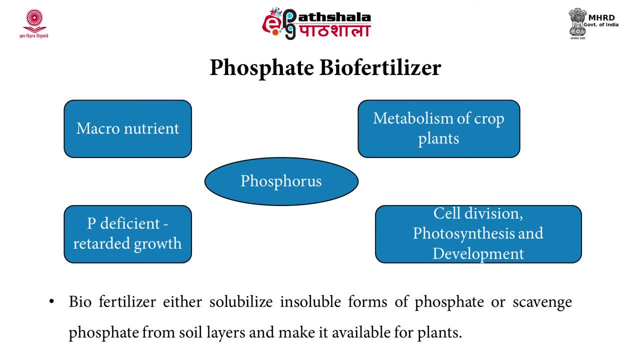 no. in turn, proper growth of the plant and plant will show a retarded growth. This phosphate bio fertilizer. it works in two ways: it either solubilize insoluble form of phosphate or it helps in it scavenge the phosphate from soil layer and make it available. 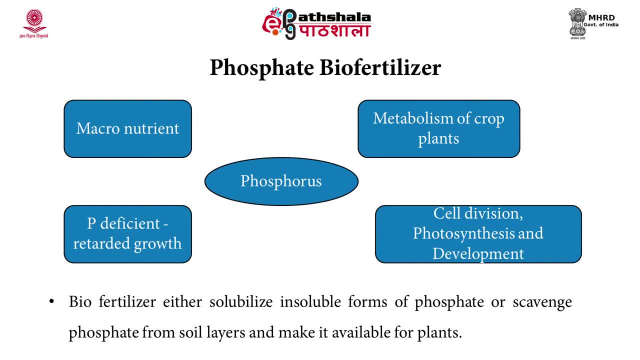 for the plant, The phosphate which is in association, which is in the associated form, in some inorganic form which is not easily available for the plant, that is being solubilized by the phosphate bio fertilizers and they make it available to the plant and for further, for good growth. 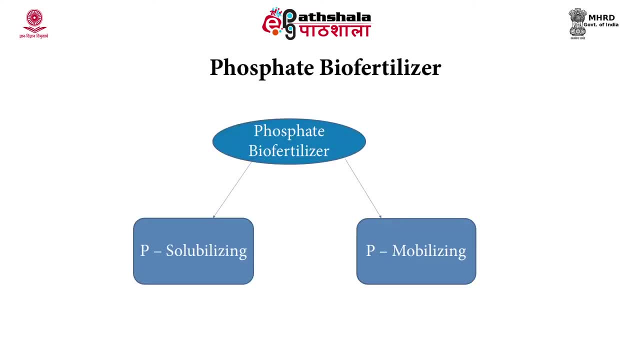 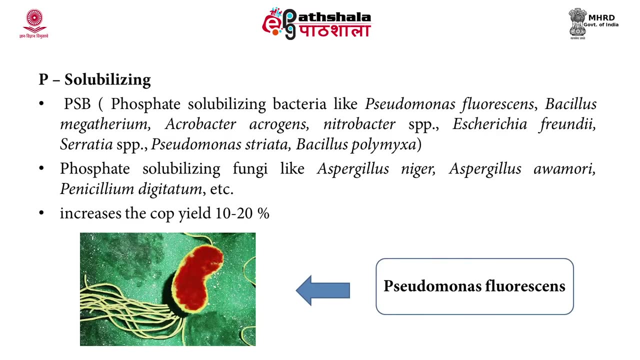 of the plant, So phosphate bio fertilizers. it is of two types: P solubilizing and P mobilizing. P solubilizing, that is PSBs, Phosphate Solubilizing Bacteria. examples of PSBs are Phosphate Solubilizing. 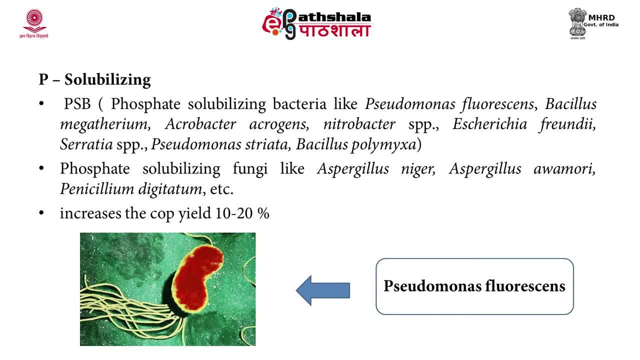 Bacteria are Pseudomonas, Bacillus Acrobacter, Pseudomonas strata and Bacillus polymyxa. What is the role of P solubilizing bacteria? What they do? they convert the inorganic form of phosphate which is present in the soil and 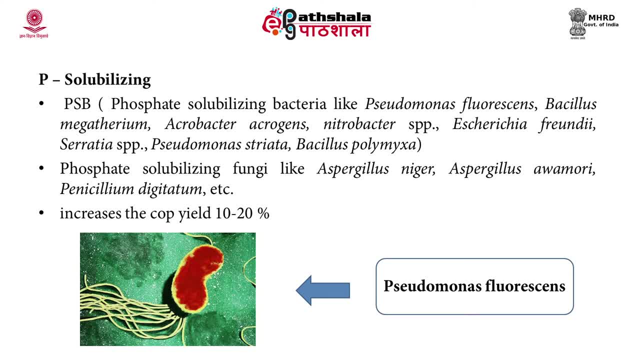 by the action of certain enzymes they convert that inorganic form into the organic form and make it available for the plant growth. Phosphate solubilizing: there are some phosphate solubilizing fungi also, such as Aspergillus niger, Aspergillus avamori and Pencilium, etc. 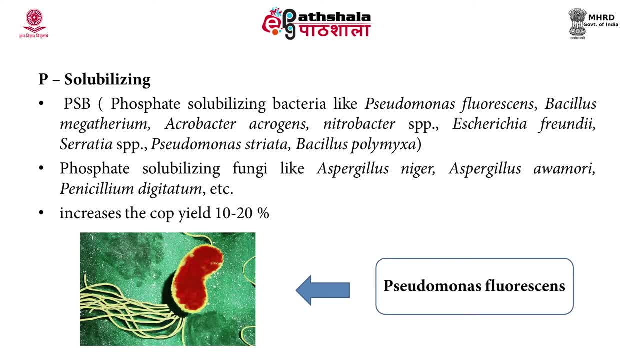 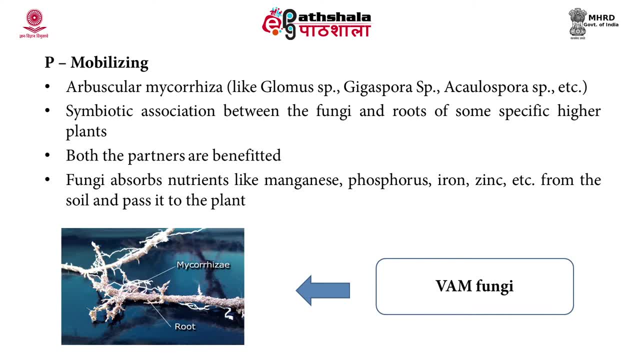 PSBs increase the crop yield by 10 to 20 percent. This is P solubilizing bacteria And The other one is P mobilizing bacteria. P mobilizing bacteria are vascular microhiza. they work in symbiotic association between fungi and root of some specific higher plants. 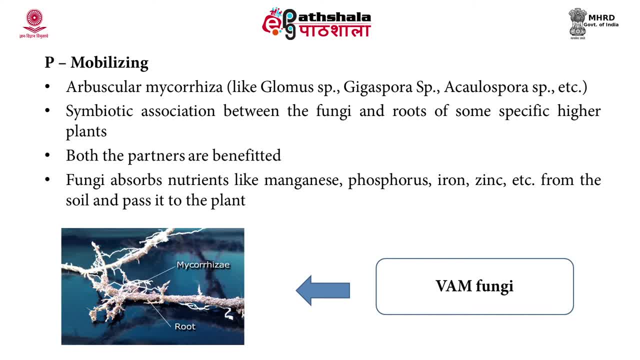 In case of PSBs that we discussed earlier. PSBs, they are not in any kind of associations. they are free living bacteria that are present in the soil, but P mobilizing bacteria. they are in symbiotic association with the fungi and root of some specific higher plants only. 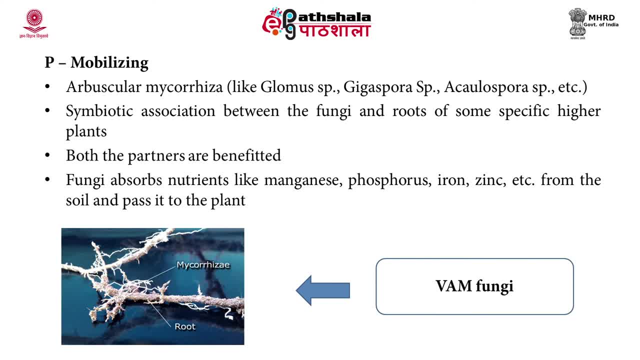 In symbiotic association means the both partners are benefited. what? what is how they function? that the fungi? they absorb nutrients like manganese, phosphorus, iron, zinc, etc. from the soil and pass it to the plant. There is no conversion process, that they are not converting any inorganic form of phosphorus. 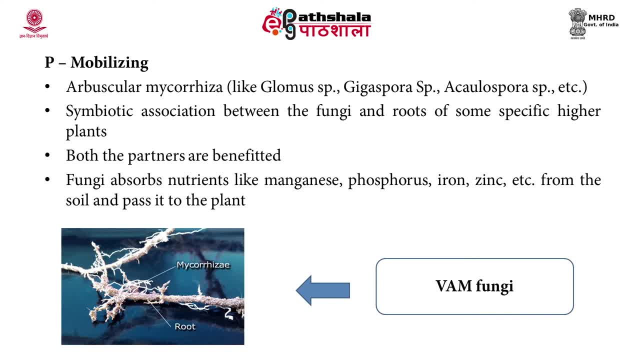 and then passing it to the plant. they are directly absorbing the available form of the plant, That which is somehow which is not easily available, And But they absorb that phosphorus from the phosphorus or the nutrients from the soil part and pass it to the plant for their further better growth. 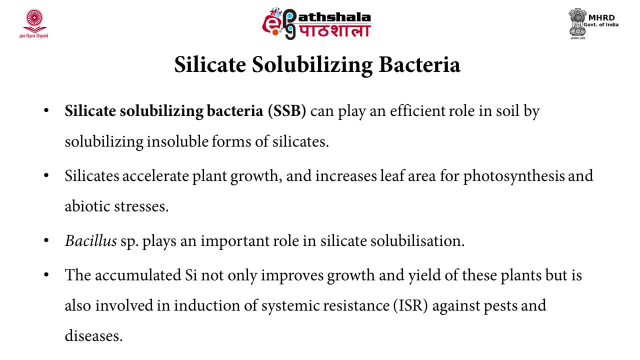 The next one is silicate solubilizing bacteria, as the name suggests that they help by. they help in solubilizing the silicate. Silicate solubilizing bacteria can play an efficient role in soil by solubilizing insoluble. 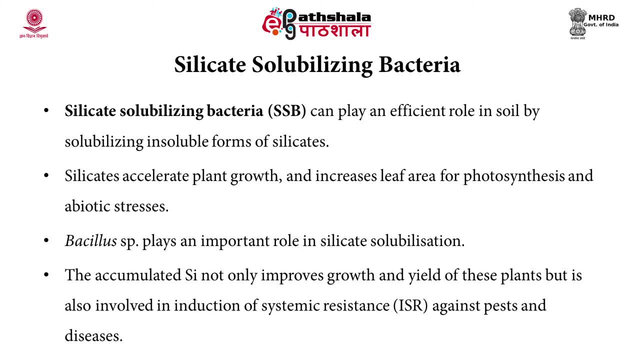 form of silicates and make it available to the plant. They also help in plant growth and they their major role is to increase by increasing the leaf area for photosynthesis. They also prepare, or we can say prepare the plant for against the resistance, or they can. 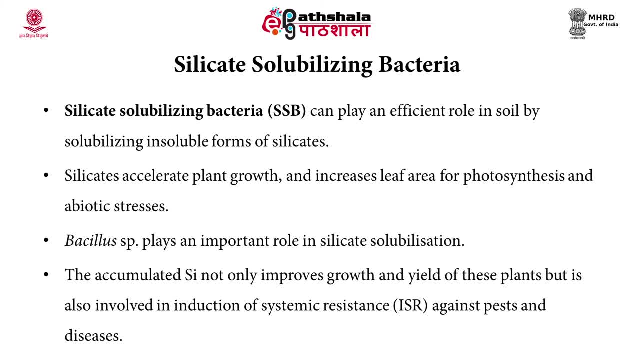 also help in help the plant against abiotic stresses, The bacillus species. it is very important. it's very important and plays a major role in silicate solubilization, The accumulator silicate is not only. it not only improves the growth And yield of the plant. 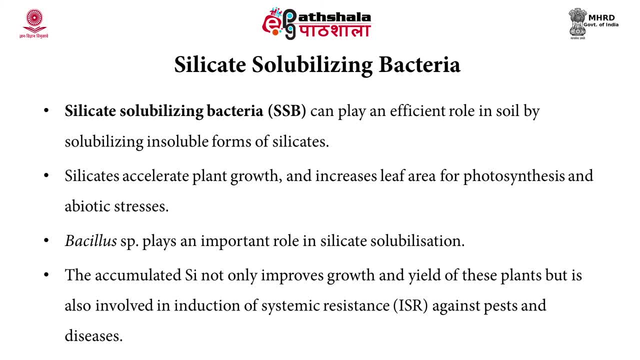 But it is also involved in the systemic resistance, as I told you that abiotic stress. it is playing its. it plays its role in against abiotic stresses and also they are not the accumulated. silicate also helps in protecting the plant against some pests and diseases. 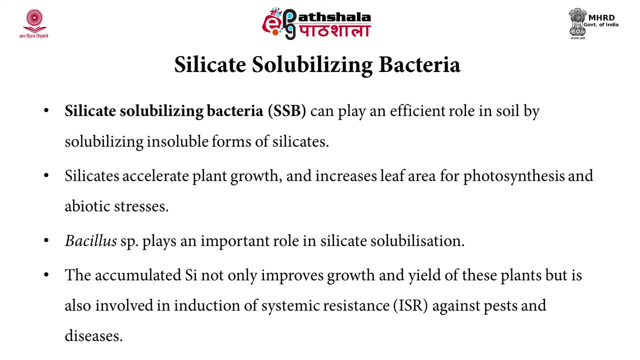 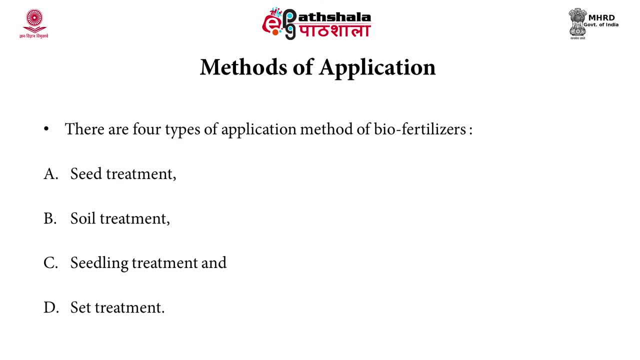 This. we discussed about the type of bio fertilizers, the three type of bio fertilizers: nitrogen, phosphate and silicate. Now now the next question is how these fertilizers are being used, the method of their application. they are basically four type of application methods of bio fertilizers. one is seed treatment. 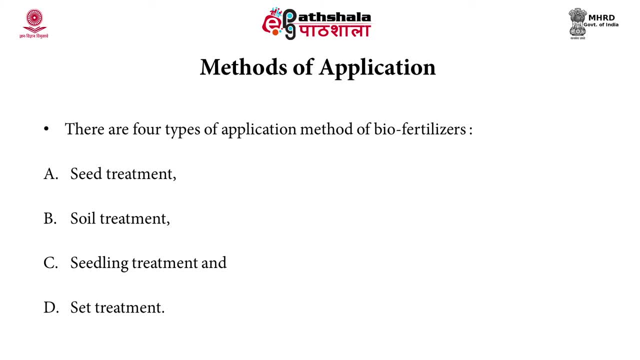 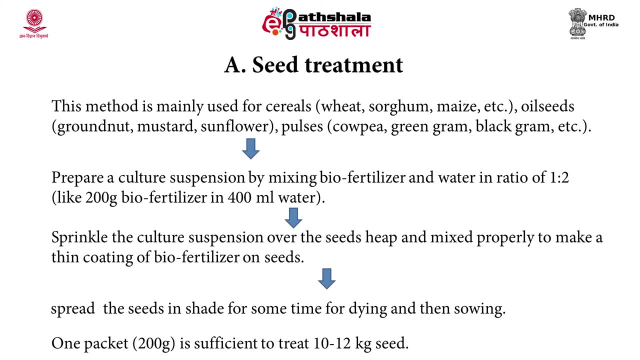 then the soil treatment, seedling treatment and the set treatment will discuss these treatments one by one. let's start with the seed treatment. Seed treatment, as the name suggests that in this treatment the bio fertilizers are being applied. They are applied directly on the seed. 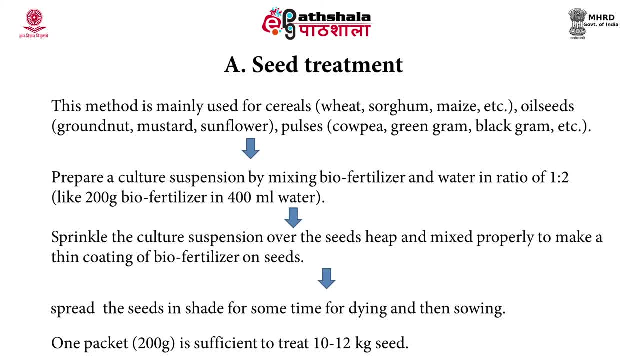 But how they are applied will discuss at what ratio they are being used. This method is used mainly used for cereals such as wheat, sorghum, maize, etc. and oil seeds and pulses. The first step of this application- how to use seed treatment- is- will prepare a culture. 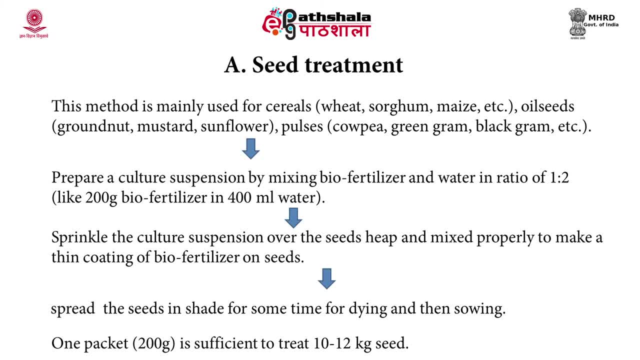 suspension by mixing bio fertilizer and water in a ratio of one is to two. For example, If we are using two hundred grams of bio fertilizer, then we will use four hundred ml of water after preparing a culture. suspension of bio fertilizer and water in ratio of one is to one. 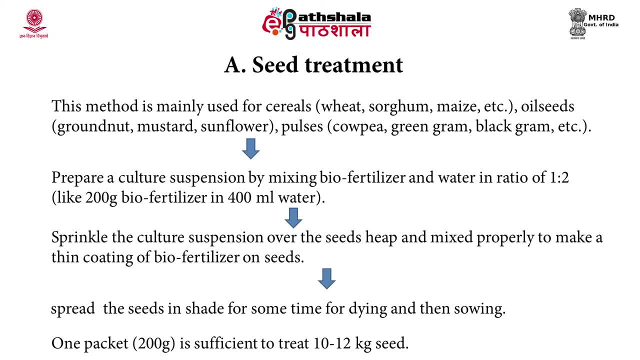 This culture suspension is spread or sprinkled over the seed heap and mixed properly to make a thin coating of bio fertilizer on seeds. These seeds are dried. the next step is to dry the seeds for some time in shade, and then the further step is sowing. 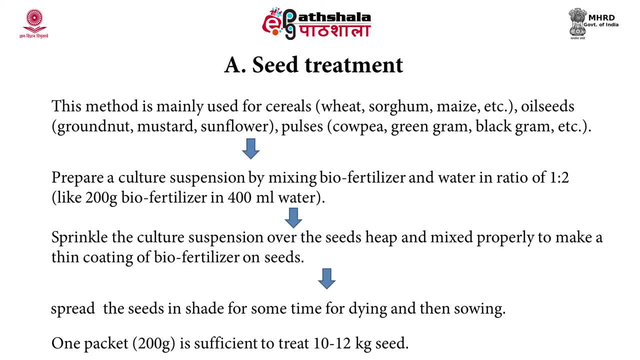 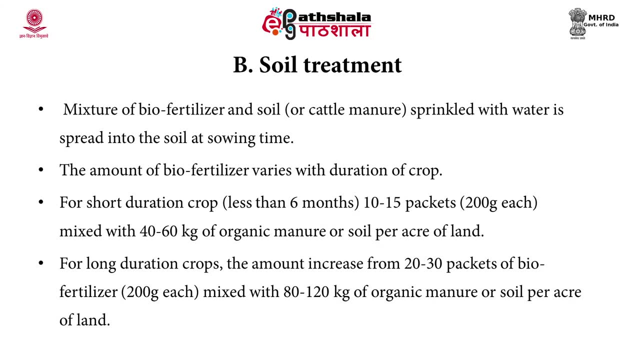 One packet Is, If we talk about the ratio, one packet of bio fertilizer. if it's of two hundred grams, it is reported that one, two hundred gram of bio fertilizer is sufficient to treat twelve, ten to twelve kg of seeds. Next application method is soil treatment. in this method, mixture of bio fertilizer and 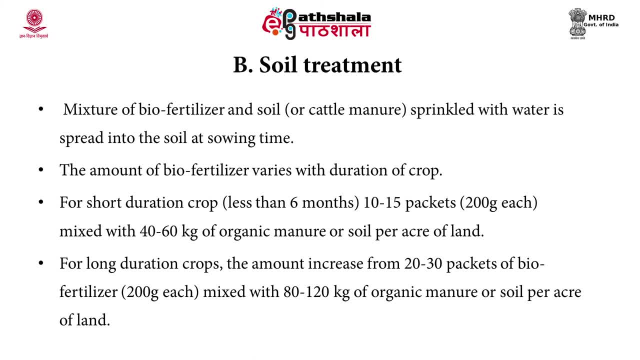 soil is prepared with the help of what we use- water, as, as we discussed earlier, that a mixture of bio fertilizer and soil- Sometimes we can use cattle manure- is sprinkled with water and spread on this on the, on directly on the soil, in in seed treatment seeds. seeds are being treated by bio fertilizer suspension. 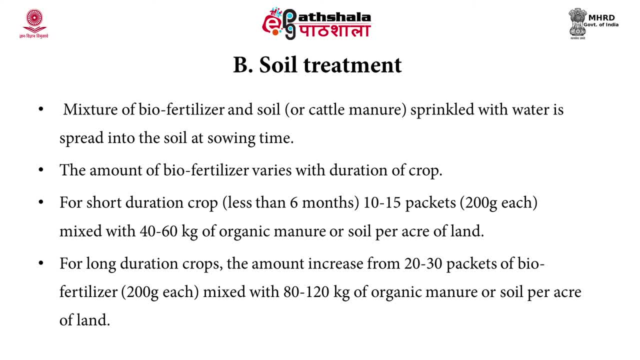 but in soil treatment we are directly applying the suspension on the soil at the sowing time. The amount of bio fertilizer varies with duration of crops. for example, if we have a short duration crop means less than six months, then ten to fifteen packets, two hundred grams each, is. 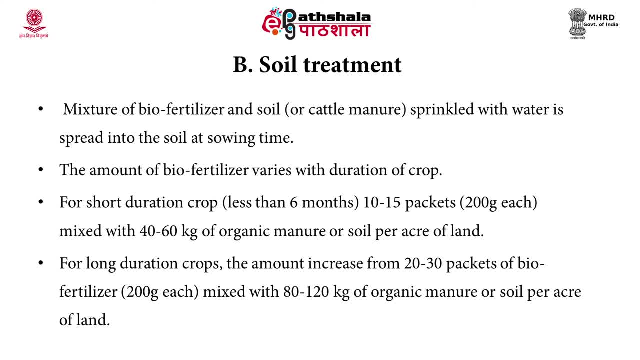 mixed with forty to sixty kg of organic manure Soil per acre of the land. if we talk about long duration, long duration crops, the amount increases from twenty to thirty packets of bio fertilizers with mixed with eighty to one twenty kg of organic manure or soil per acre of the land. 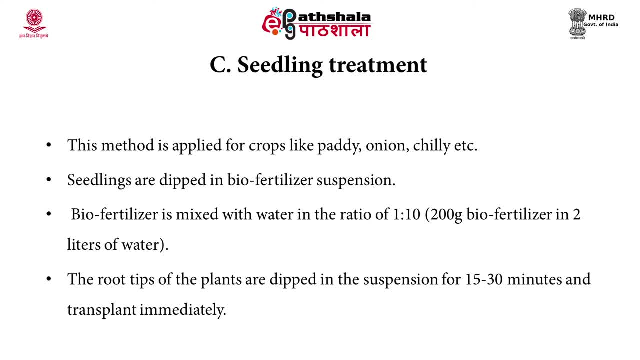 The next treatment is seedling treatment. This method is applied for crops like paddy, onion, chili, etc. Because the seedlings- they are suspension- is prepared in similar way that the bio fertilizer is mixed with water in ratio of one is to ten. In seed treatment we mix the. the ratio was one is to two, but here the ratio is one is. 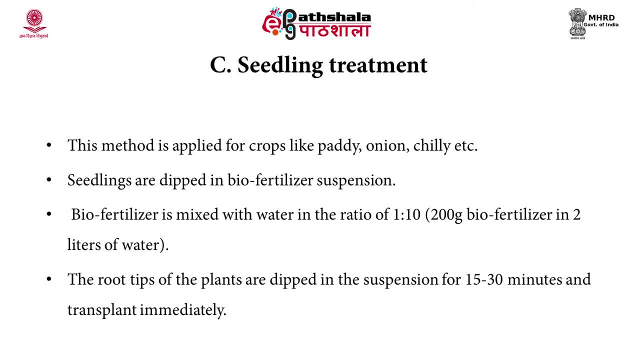 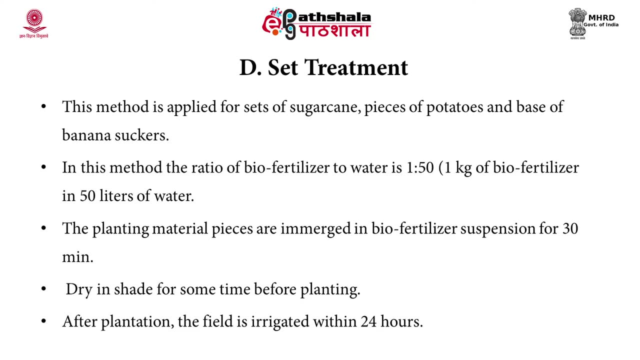 to ten the seedlings. the suspension is prepared. then the seedlings are dipped in bio fertilizer suspension for thirty minutes. then the root tips of the plants that we have already dipped- they are transplant immediately. There is no drying step in the seedling treatment. Next is set treatment. 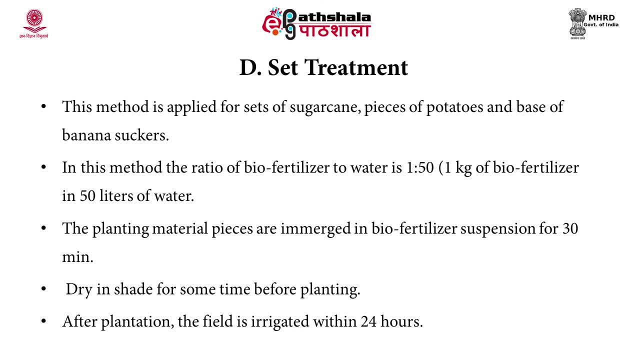 Set treatment is applied for the set of sugar canes of reuse for the crops like sugar cane, pieces of paddy potatoes, base of banana suckers, etc. In this method the ratio of biofertilizer to water is 1 is to 50, 1 is to 50 means 1. 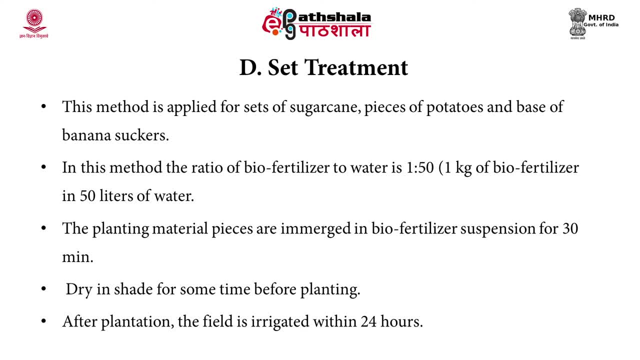 kilogram of biofertilizer in 50 liters of water. The planting material pieces are immersed in the biofertilizer suspension for 30 minutes. Next step is to dry them in shade for some time before planting. The important step is that after plantation, the field is irrigated within 24 hours. 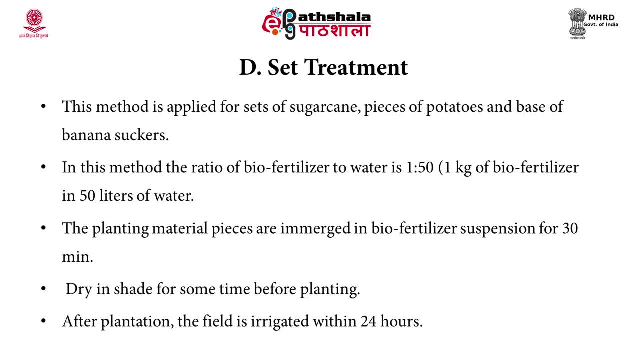 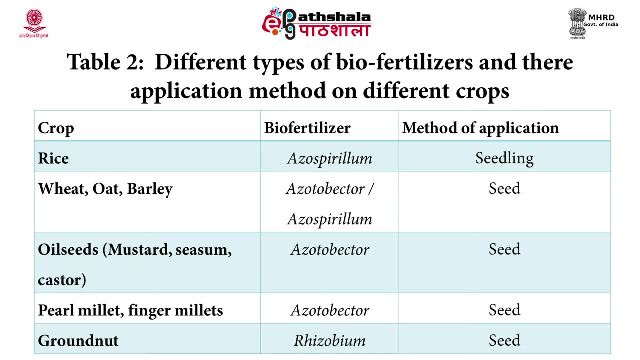 It's very necessary step to irrigate the fields after plantation within 24 hours. This table describes that. we discussed earlier the different methods of application. This is a summary of that application method: Different types of biofertilizer and their application method on different crops. 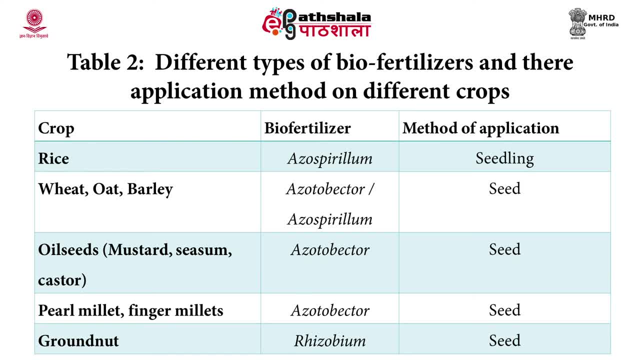 For example, rice. the method of application is seedling, means the root tips are being, the tips are being dipped in the biofertilizer suspension and then transplanted and then plantation was done, Then the soybean seed treatment is used. 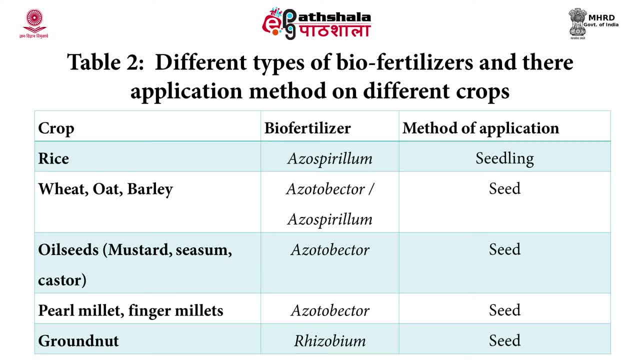 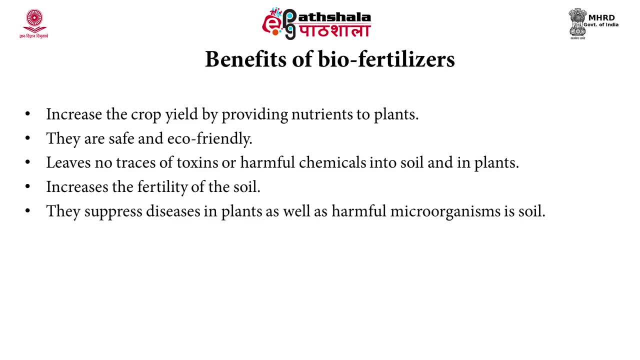 The seeds are being. they're being coated with the biofertilizer suspension, then dried for some time in the shade, and therefore the sowing step was followed. Next is benefits of biofertilizers. Biofertilizer increase the crop yield by providing nutrients to plants. 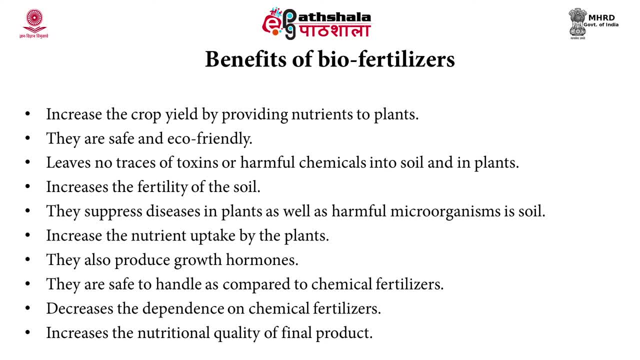 They are safe and eco-friendly. The leaves no traces of toxins and harmful chemicals into soil and in plant. Biofertilizer helps in increasing the fertility of plants. Biofertilizer helps in increasing the fertility of plants. Biofertilizer helps in increasing the fertility of soil. 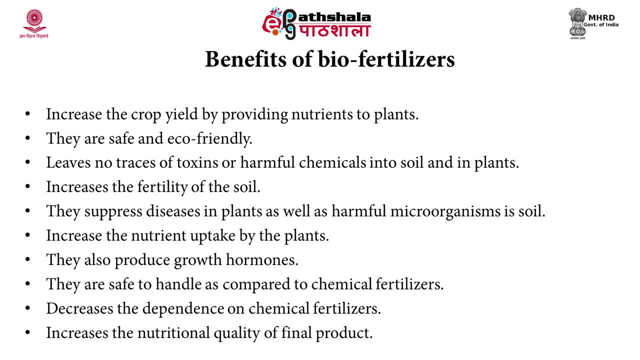 This suppress disease in plant as well as harmful microorganism in the soil. Biofertilizer increase the nutrient uptake by the plant by making the non-available. by making nutrients available to the plant, They also produce growth hormones. They are safe to handle as compared to chemical fertilizers. 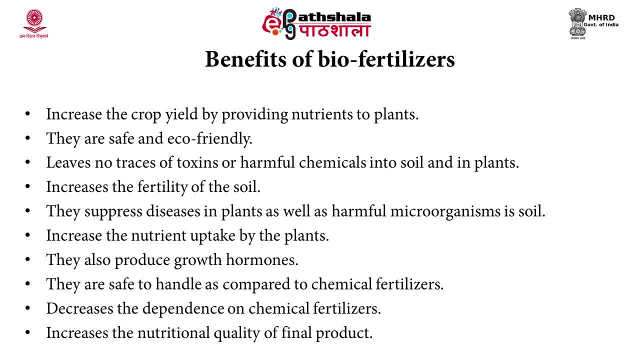 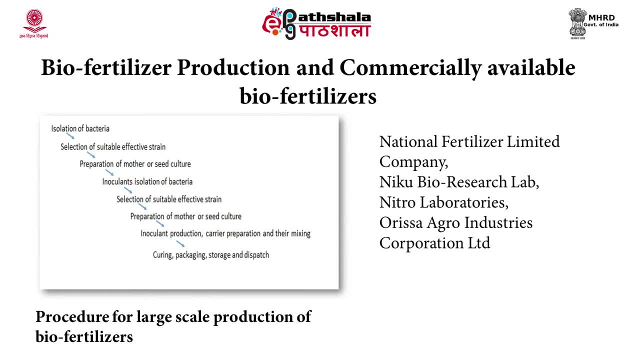 They decreases the dependence on the chemical fertilizers, as chemical fertilizers are not that much safe. They increase the nutritional quality of the final crop. Biofertilizers increase the environmental value of the final product. We discussed about the types of biofertilizers and methods of application. 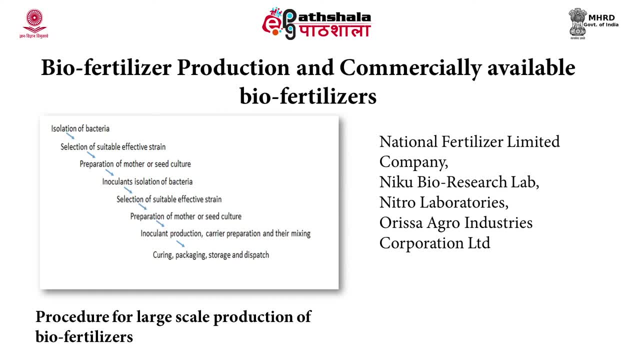 Now how bio fertilizers are produced commercially. Before starting with the production at the commercial level, we will discuss and how we will continue to the production phaseぁ. We will discuss this step by step and sometimes you may ask them: what is that we are discussing? 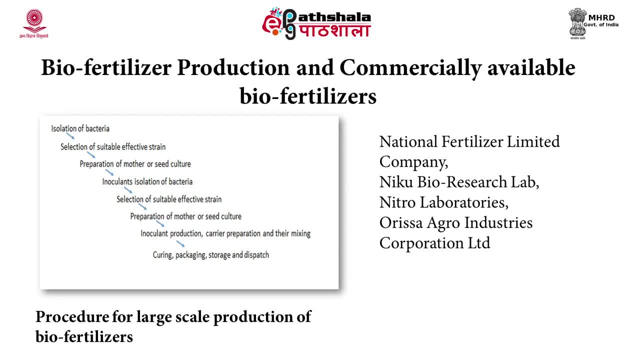 in the conversation. they say it is isolation of the bacteria. Fortunately, bacteria rotational process is capable of making consumers plants grow faster. but the most important, that the cảm дивor בב, Layer 2, the bacteria which is capable, which has the potential of having the bioFertilizer potential. 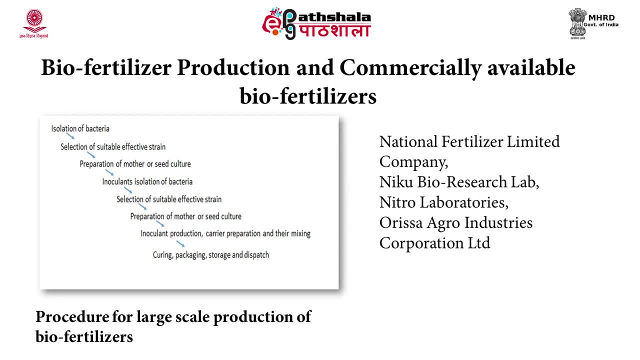 and it is in the accumulations for which the plant can be grown. Agro nutrients level is become 5 square and if there are some which may not be observeable, but we will discuss this short path by which to, for example, improve the crop size. 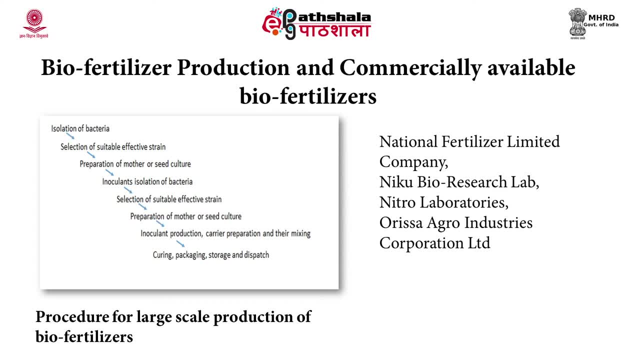 the isolation part was done, then the next step is to select the suitable effective strain in bio fertilizer production or the commercial production. it's very important to know that the that strain should be non pathogenic. we can't go for the pathogenic strains, so this is an 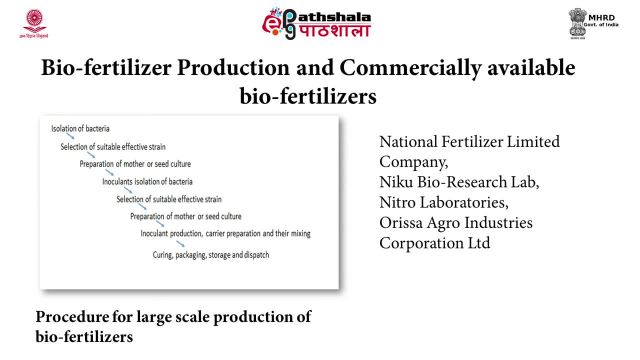 important step for bio fertilizer development. X isolated bacteria is inoculated in the suitable bacteria in the suitable culture. preparation of mother or seed culture. it was done at commercial level then the then we cannot apply bio fertilizer or microorganism directly to the field. they need some career for with with the help of career we can only apply them in the field. so career. 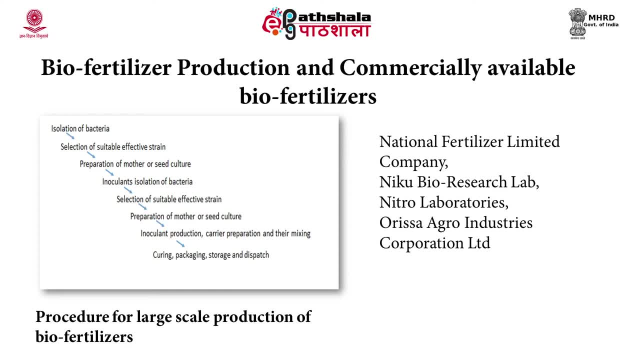 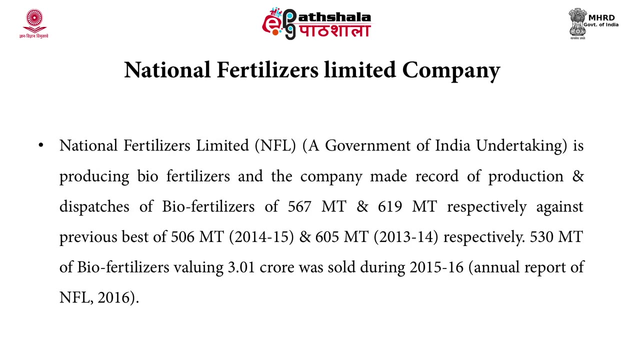 preparation and their mixing was done. the next step is packaging and storage and then dispatch to the market. there are some bio fertilizer producing companies. few of them are mentioned here- that the national fertilizer limited, Niku bio research lab, nitro laboratories and Orissa agri industries corporation limited. the national fertilizer limited company, NFL. 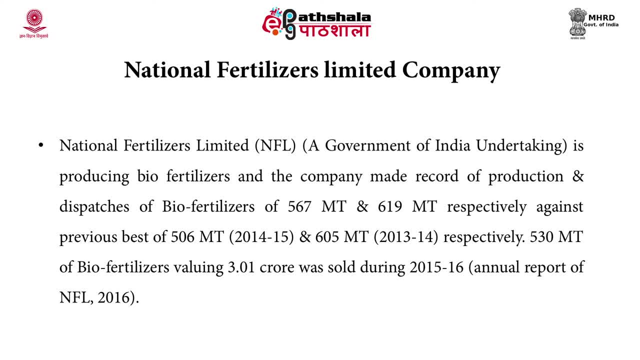 it is a government of India undertaking body and is producing bio fertilizer, and this company made a record of production and dispatch of bio fertilizer of 567 metric and 619 metric ton respectively, against the previous best of 506 metric ton in the year of 2014-15 and 605 metric ton in 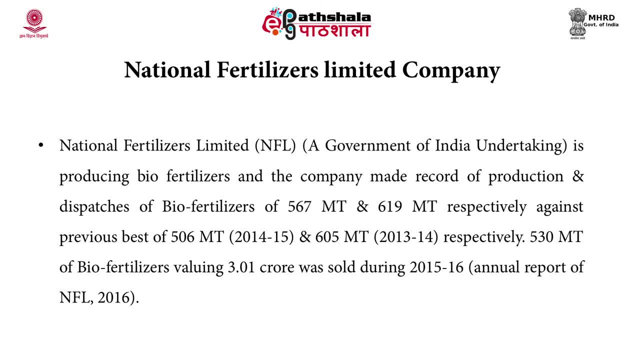 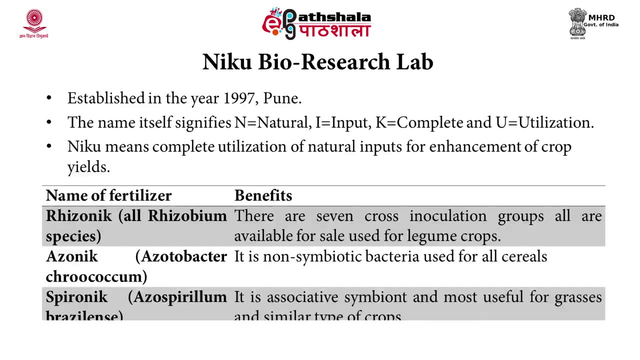 the year of 2013-14, respectively 530 metric ton of bio fertilizer value- about around 3.01 crore, and it was sold during the 2015-16, as mentioned in the annual report of NFL 2016.. Niku bio research laboratory. 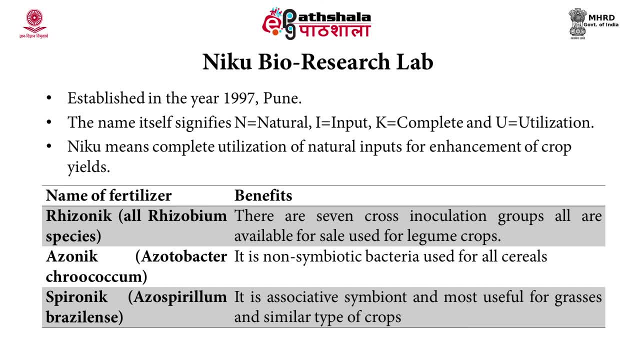 this lab was established in the year 1997 in Pune, as the name suggests itself that N for natural, I for input, K stands for complete and U stands for utilization, which means complete utilization of natural inputs for enhancement of crop yields. this table shows the bio fertilizer that that 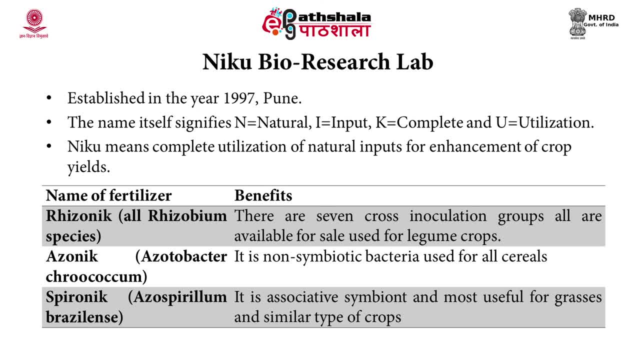 are produced at Niku bio research lab and their benefits also. for example, they are producing rhizonic- the brand name is rhizonic or- which is used against all the rhizobium species. the azonic, the azotobacter formulation, is being used in the azonic bio. 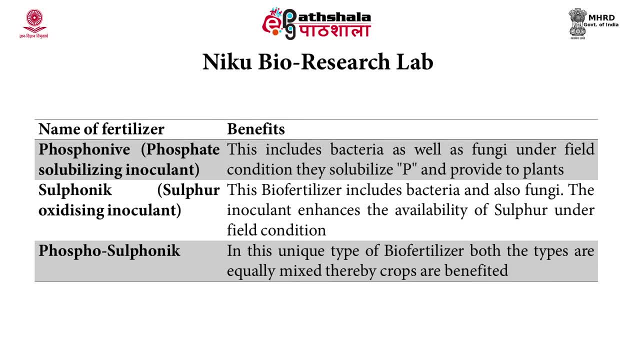 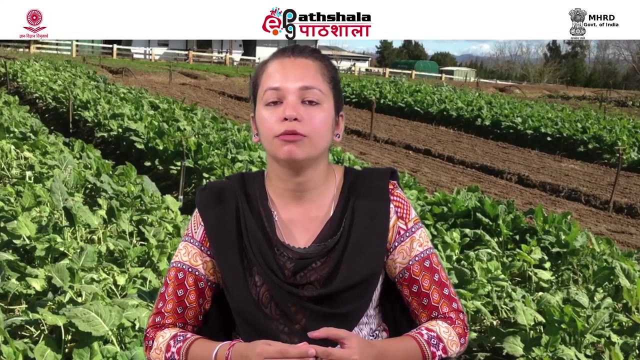 fertilizer, the phosphonib, that is, phosphate solubilizing inoculant, which is the suspension of phosphate solubilizing bacteria, sulfonic, as name suggests that a sulfur oxidizing inoculants are used in financial proof. terceric acid insulation on wanting to continue their Libraries of nau między.